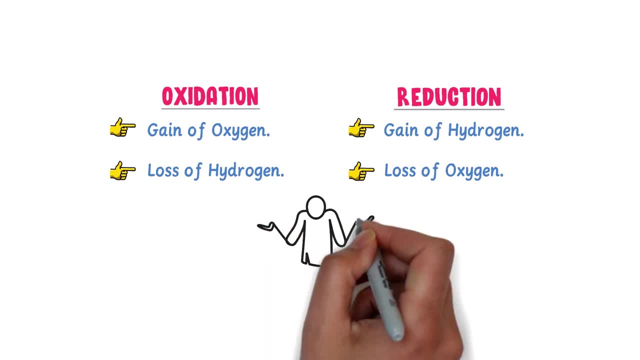 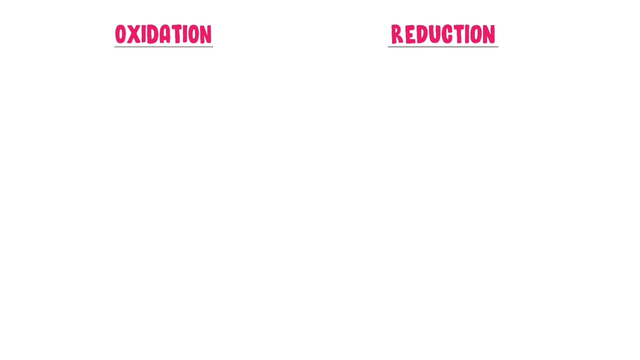 and loss of oxygen. Personally, I do not teach oxidation and reduction like this, and I will give you the reason at the end of this lecture. Now let me teach you the basic and easy concept of oxidation and reduction reactions. The common mnemonic used for oxidation and reduction is: 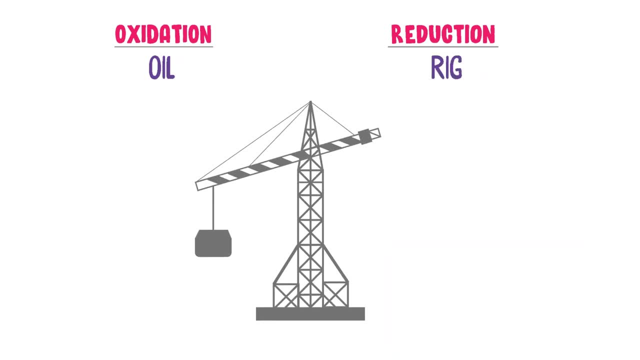 oil rig. It is an instrument which is used for drilling an oil well. The oil stands for oxidation is loss of electrons. The rig stands for reduction is gain of electrons. So note it down that oxidation is the loss of electrons and reduction is the gain of electrons. 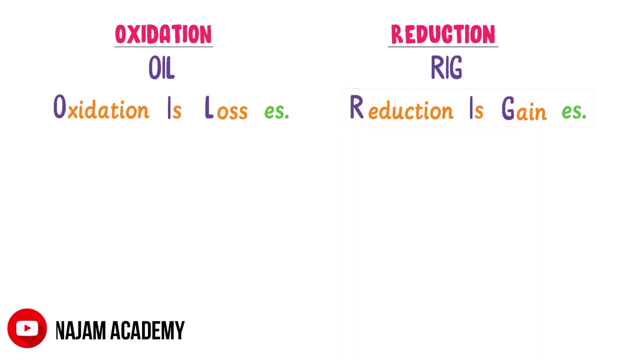 For example, consider sodium atom and chlorine atom. Now sodium loses one electron and chlorine gains one electron. After losing one electron, sodium becomes a positive iron and chlorine gain this electron to become a negative iron. Sodium has lost one electron, so it is oxidised. 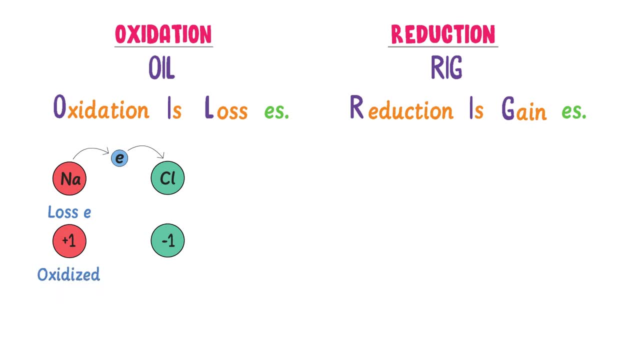 Chlorine has gained one electron, so it is oxidised enough to return positive iron When cylinder it is reduced. Finally, we get sodium chloride, which is commonly known as a table salt. Secondly, consider potassium atom and hydrogen atom. Now, potassium atom loses one electron. 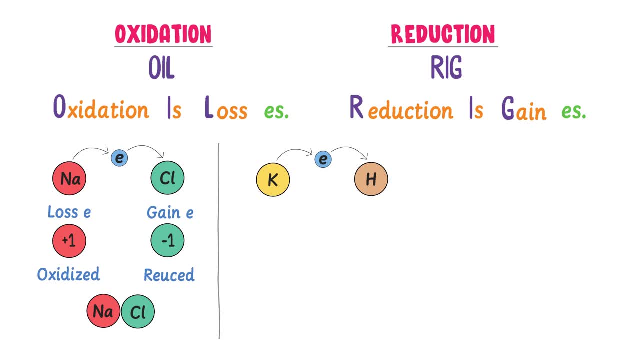 and hydrogen. atom gains this electron. After losing one electron, potassium becomes positive ion and hydrogen becomes negative ion after gaining one electron. Potassium has lost one electron, so it is oxidized. Hydrogen has gained one electron, so it is reduced. Finally, we get 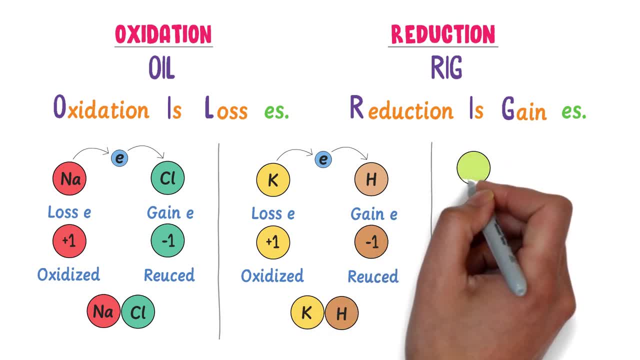 potassium hydride. Thirdly, consider magnesium atom and bromine atom. Now, magnesium loses two electrons because its valency is two. Bromine atom can accommodate only the hydrogen atom and the hydrogen atom can accommodate only the hydrogen atom. Bromine atom has only one electron, hence we need one another bromine atom to accommodate the second. 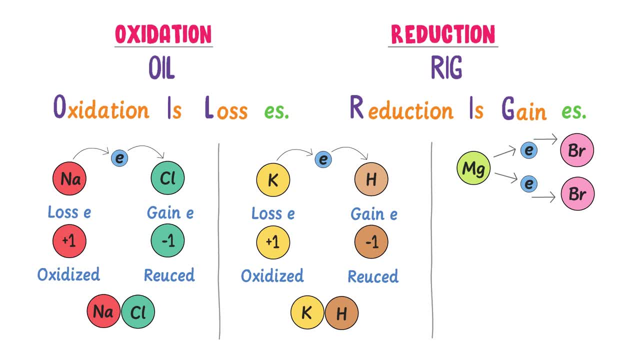 electron of magnesium. After losing electrons, magnesium becomes double positive ion and each atom of bromine becomes negative ion. after gaining one electron, Magnesium has lost two electrons, so it is oxidized. Bromine atoms gained electrons, so they are reduced. Finally, we get magnesium. 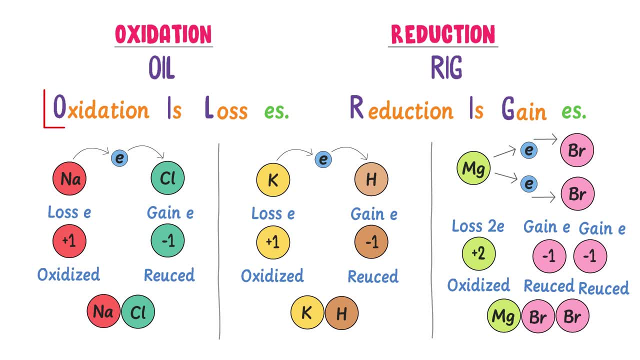 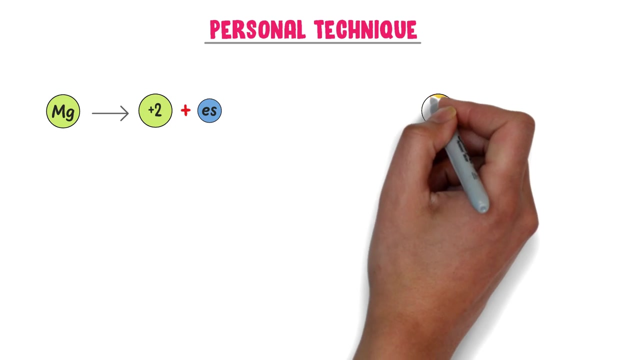 Therefore, remember that oxidation is the loss of electrons like sodium, potassium and magnesium lose electrons, while reduction is the gain of electrons like chlorine, hydrogen and bromine gain electrons. Now let me teach you my personal technique of learning oxidation and reduction. Consider magnesium atom and magnesium ion, bromine atom and bromine ion. We can see that 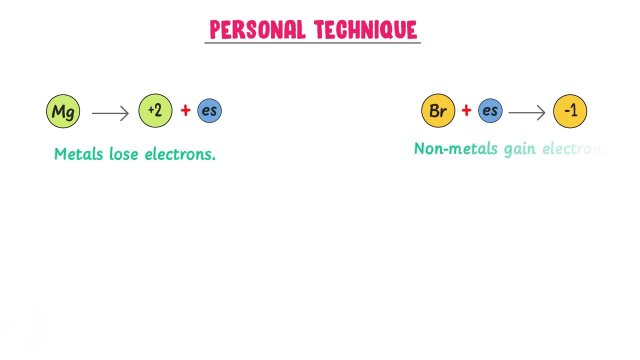 metals lose electrons and non-metals gain electrons. For example, magnesium atom is a neutral particle, so the net charge on it is zero. Later, when magnesium atom loses two electrons, it becomes ion, having double positive charge. This apparent charge on magnesium atom and 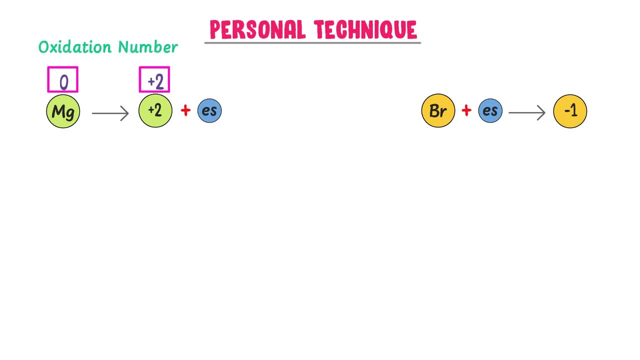 magnesium ion is called oxidation number or oxidation state. Also, the oxidation number of bromine atom is zero. So the oxidation number of bromine atom is zero and the oxidation number of bromine ion is negative one. Now listen carefully. Oxidation number of magnesium increased from zero. 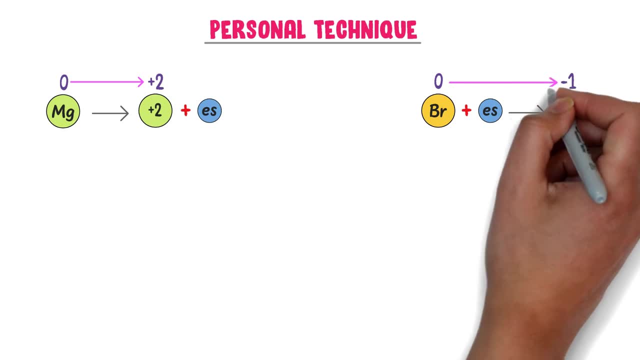 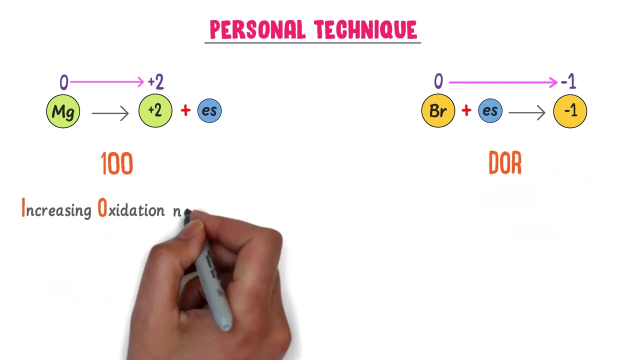 to positive two, while oxidation number of bromine decreased from zero to negative one. Here comes the climax of this lecture. I teach to my students my personal mnemonic as 100 DOOR. 100 stands for increasing oxidation number is oxidation. DOOR stands for decreasing oxidation number is reduction. 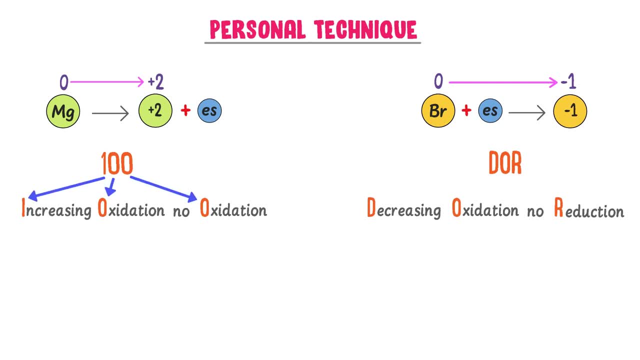 Remember that in 100, 1 stands for I and 00 stands for 00 and DOOR stands for decreasing oxidation. number is reduction Here. magnesium is oxidized because it has lost electron and its oxidation number increased from zero to positive two, while bromine is reduced because it has gained. 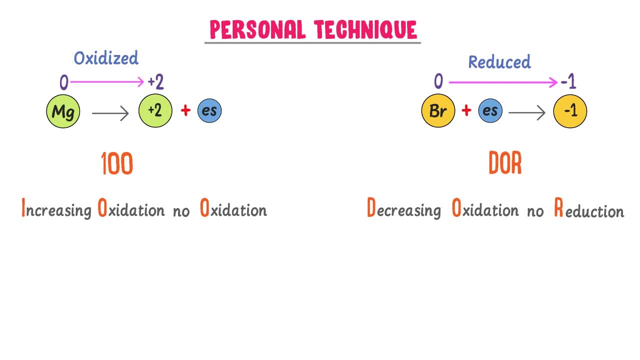 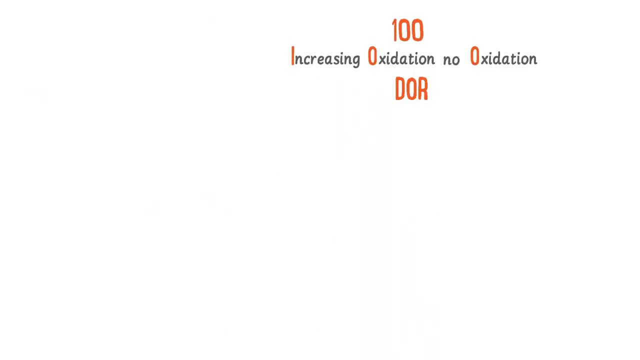 electron and its oxidation number decreased from zero to negative one. Now I will show you the power of this trick. in order to find the oxidation and reduction reactions, Firstly, I write 100 DOOR. I mean increasing oxidation- number is oxidation- and decreasing. 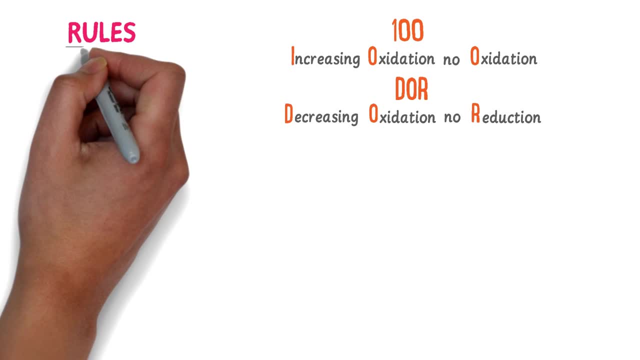 oxidation number is reduction. I write these four rules for oxidation number at one corner. If you do not know how to calculate oxidation, then you can do it by solving this matrix problem. So far, I have given you how to write the number of oxidation and reduction reaction. If you do not know how to calculate oxidation number, is oxidation and decrease oxidation number. 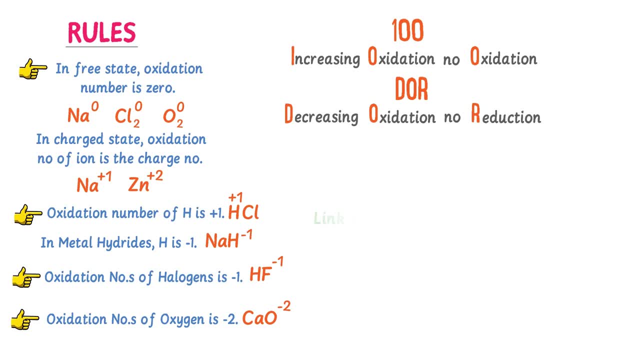 oxidation number. watch my previous lecture and its link is given in the description. the first reaction is carbon plus oxygen to form carbon dioxide gas. as we know that oxidation number in free state is zero, for example, the oxidation number of carbon is zero and that of oxygen is zero. what about the oxidation? 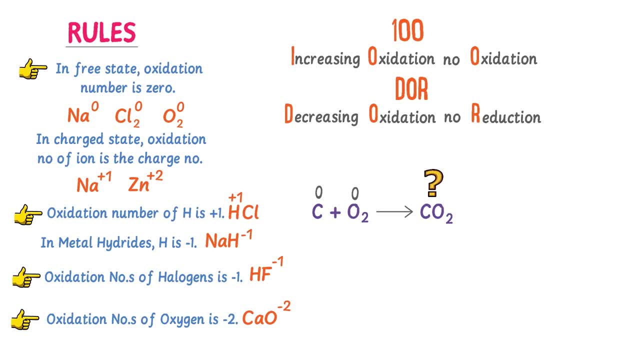 number of carbon and oxygen and carbon dioxide are combined state. well, let me calculate it. the net charge on carbon dioxide gas is zero, so the sum of all oxidation numbers must be equal to zero. I write: carbon plus 2o is equal to zero because there is one atom of carbon and two atoms of oxygen present, and carbon. 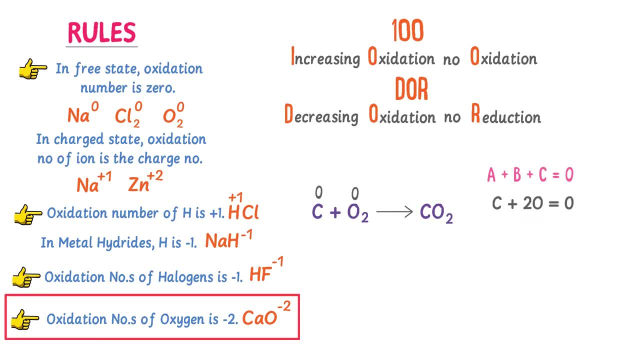 dioxide. we know that the oxidation number of oxygen and its compound is negative 2, so I put it: instead of this oxygen, I write carbon plus 2 and 2. negative 2 is equal to zero. our carbon minus 4 is equal to 0. our carbon is equal to positive 4. thus the oxidation number of 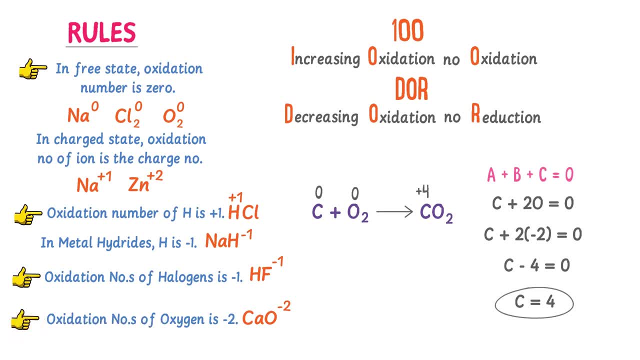 carbon is positive 4 and that of oxygen is negative 4. now listen carefully. the oxidation number of carbon increased from 0 to positive 4, so it is oxidized, while that of oxygen decreased from 0 to negative 4, so it is reduced. this reaction is called redox reaction because 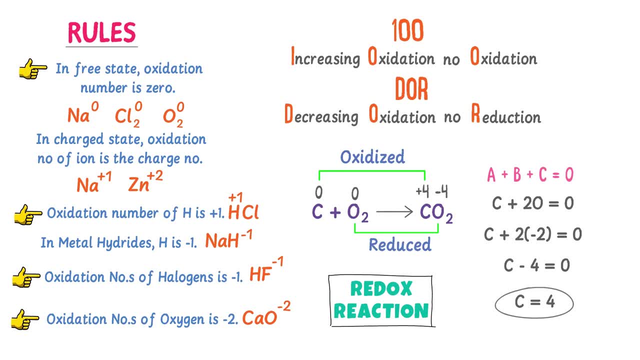 oxidation and reduction takes place in it. secondly, consider n2 plus h2 react to form Ammonia NH 3. we know that the oxidation number of any atom in free state is 0, so the oxidation number of nitrogen is zero, and that of hydrogen is also zero. now what about the oxidation number of nitrogen? 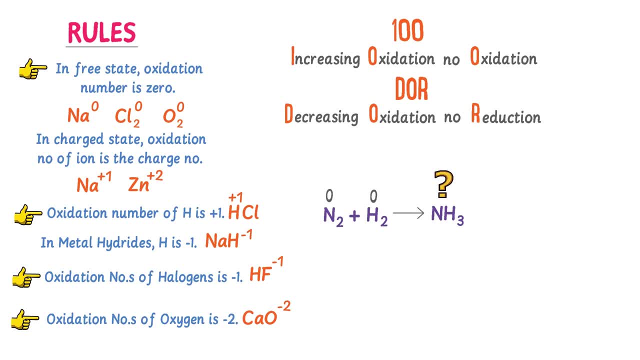 and hydrogen in combined state, NH3.. Well, ammonia, NH3 is a neutral molecule, so the sum of all the oxidation number must be equal to 0. I write: N plus 3H is equal to 0, because there is one atom of nitrogen and three atoms of hydrogen present in NH3. We know that the oxidation number of 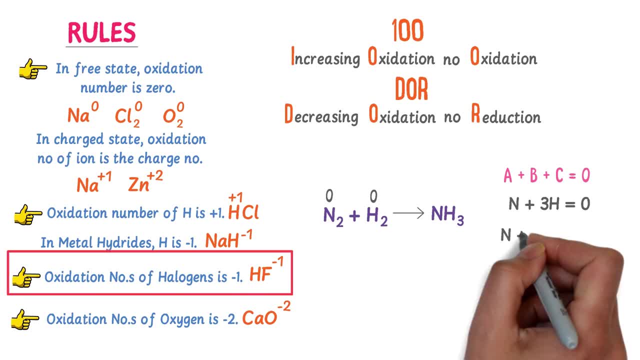 hydrogen and its compound is positive 1. so N plus 3N to positive 1 is equal to 0, or N plus 3 is equal to 0 or N is equal to negative 3.. Thus the oxidation number of nitrogen is negative 3 and. that of hydrogen is positive 3.. We can see that the oxidation number of nitrogen decreased from 0 to negative 3, so it is reduced. Secondly, the oxidation number of hydrogen increased from 0 to positive 3, so it is oxidized. This reaction is a redox reaction. 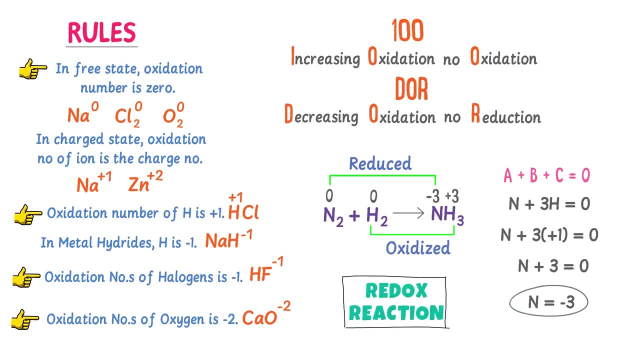 because oxidation and reduction reactions take place in it. Thirdly, let me quickly teach you two examples of decomposition reactions. Consider mercury oxide when heated decomposes to mercury plus oxygen gas. According to this rule, mercury and oxygen are in free state, so the oxidation number of mercury is zero and that of oxygen is also zero. According to this, 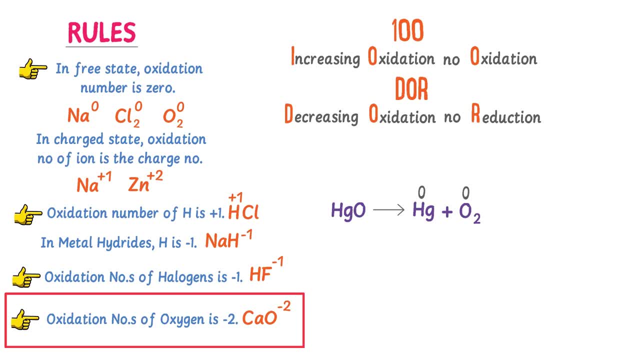 rule and combined form, the oxidation number of oxygen and its compound is negative 2.. If the oxidation state of oxygen is negative 2, then that of mercury must be positive 2, because negative 2 and positive 2 would cancel each other to neutralize this molecule. Here the oxidation, 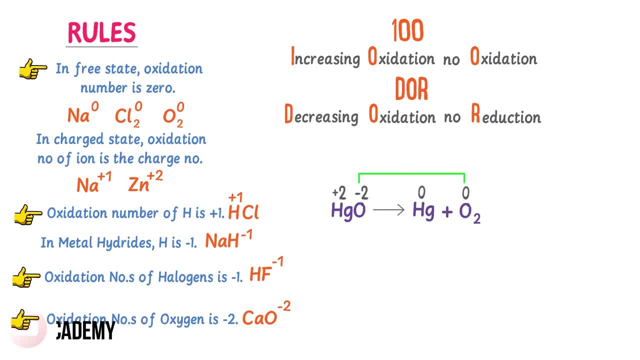 number of oxygen is negative 2 and that of mercury is positive 2.. So the oxidation number of oxygen is reduced from 0 to negative 2, so it is reduced, While that of mercury increased from 0 to positive 2, so it is oxidized. This is also a redox reaction. Lastly, consider calcium carbonate When it is. 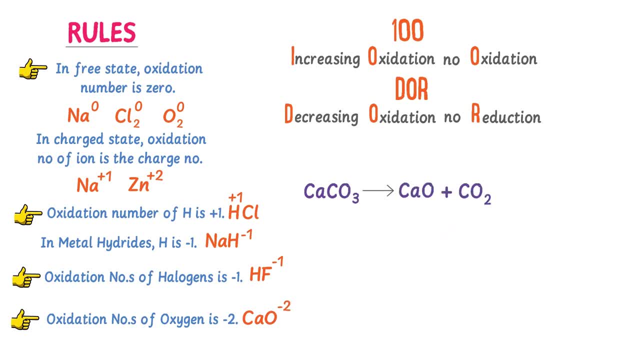 heated, it decomposes to calcium oxide and carbon dioxide gas. In case of carbon dioxide gas, we know that the oxidation number of oxygen is negative 2 and that of oxygen is also negative 2 and that of oxygen is reduced When the oxidation number of oxygen is positive 2. we understand that there are two of them acting. 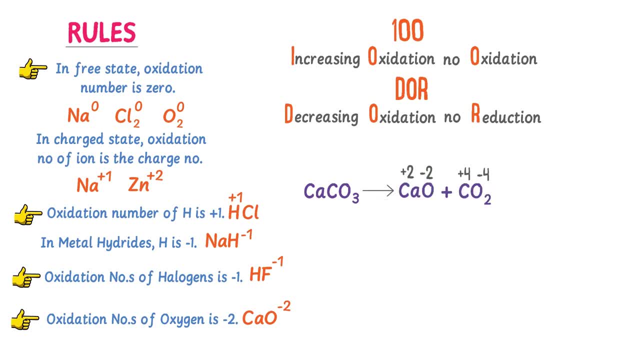 費 x ỏi r p x x. Now what about the oxidation number of carbon and calcium carbonate? Well, let me calculate it. Calcium plus carbon plus 3O is equal to zero. The oxidation number of metals like calcium is its group number or valence electrons. 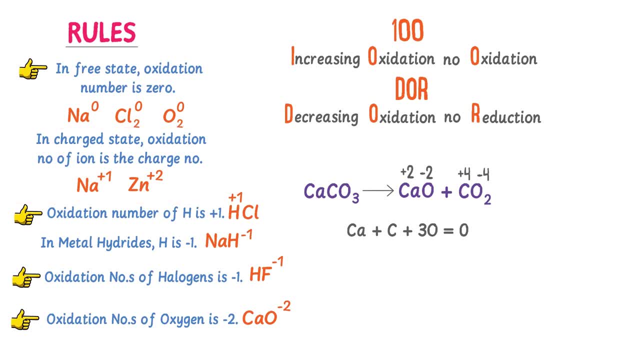 We know that calcium atom is present in second group, so its oxidation number is positive, 2.. C plus 3 and that of oxygen is negative. 2 is equal to zero. So I get 2 plus C minus 6 is equal to zero, or C is equal to positive 4.. 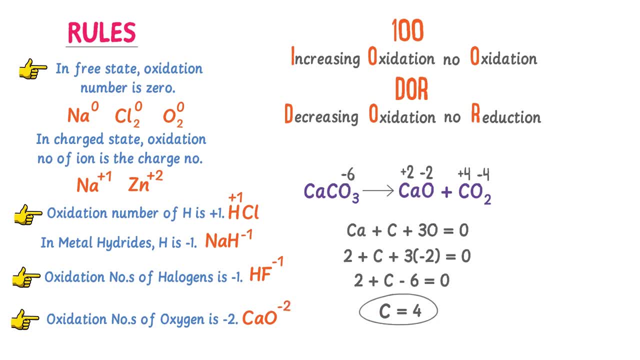 Thus, the oxidation number of oxygen is negative- 6, that of calcium is positive- 2 and that of carbon is positive- 4.. Now listen carefully. the oxidation number of calcium does not change and remains positive 2.. The oxidation number of carbon does not change and remains positive- 4.. 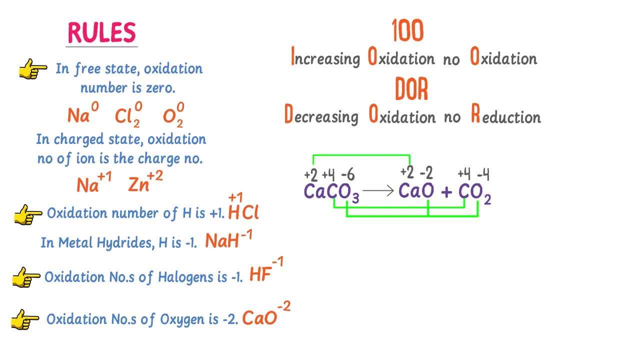 And the oxidation number of oxygen does not change and remains negative 6. So we say that no oxidation and reduction reactions take place in this reaction. hence it is not a redox reaction. Thus, remember that a reaction may be redox or not a redox reaction depending upon oxidation. 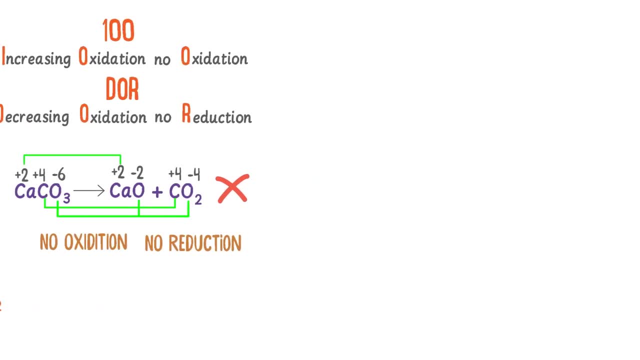 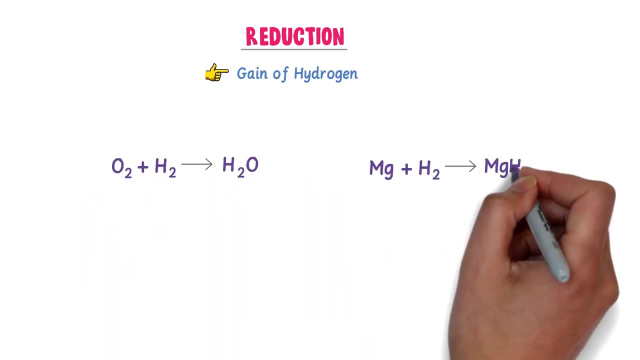 and reduction. Finally, let me show you another example. Let me show you that why I do not teach the reduction as gain of hydrogen, For example. consider these two reactions. In this reaction, oxygen gains hydrogen to form H2O. hence oxygen is reduced and hydrogen 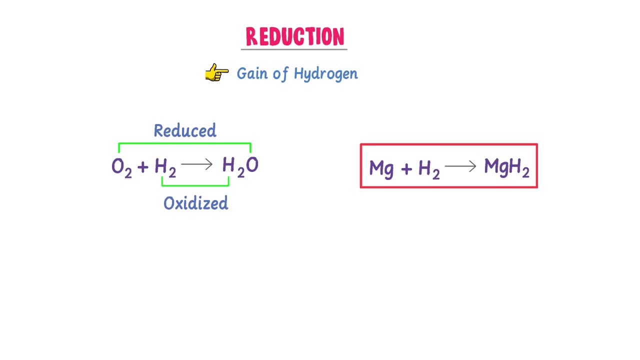 is oxidized, While in this reaction magnesium gain hydrogen to form magnesium hydride. hence magnesium is oxidized and hydrogen is reduced. So, according to this definition, the oxidation number of oxygen is negative 2. Therefore, I do not teach reduction and oxidation like this. I hope that you have learnt all about oxidation and reduction reactions. I hope that you have learnt all about oxidation and reduction reactions.